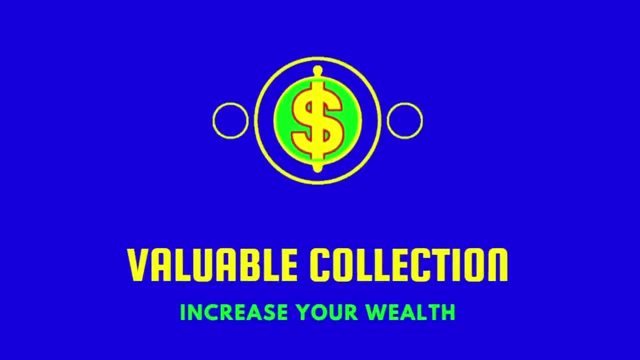 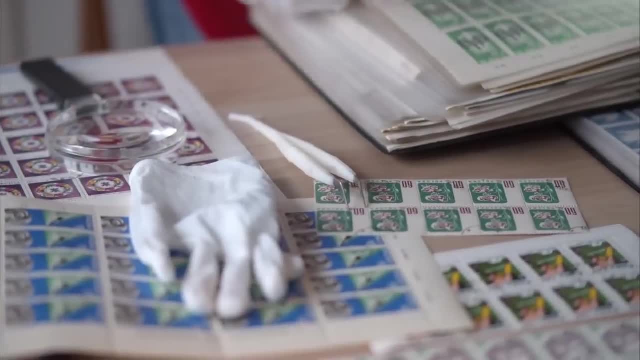 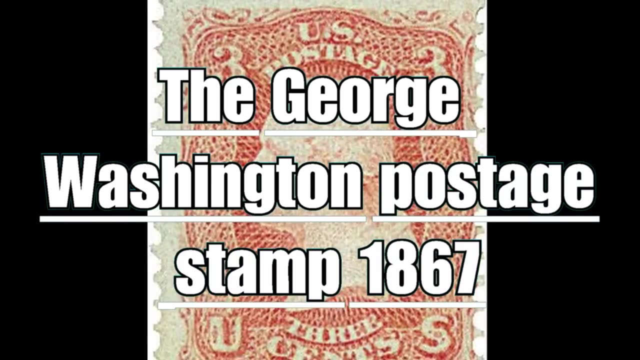 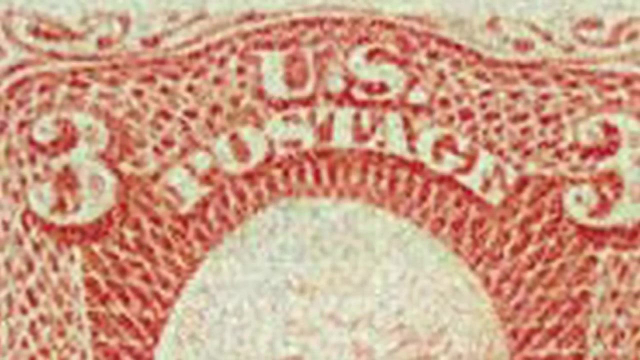 American Stamps of Rare Value Stamps proved to be an alternative investment returns that in the long term can have a very high value. The George Washington postage stamp 1867 is in orange print. it represents the face of the first president of the United States of America. at the top the inscription US postage. 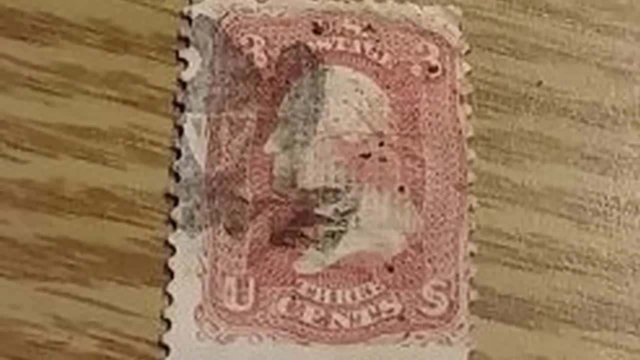 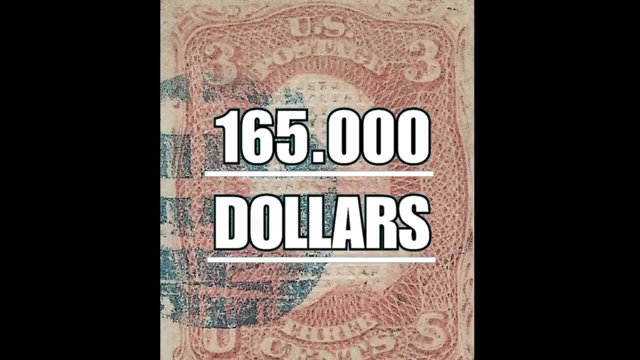 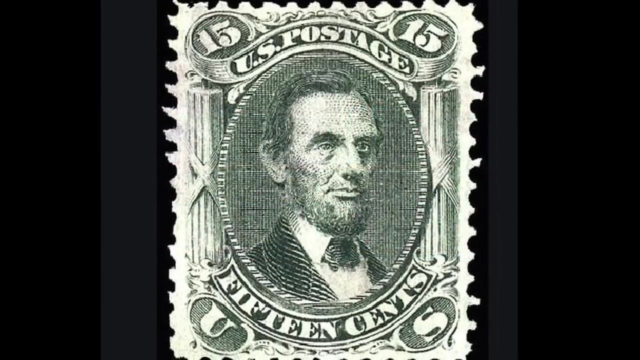 and the numbers 3, while under the face the writing of the face value of the stamp, or 3 cents, Printed in only 1,000 copies. only 4 exist today and are worth about $165,000 each. The 1867 Abraham Lincoln stamp is extremely rare and features distinctive horizontal rather than 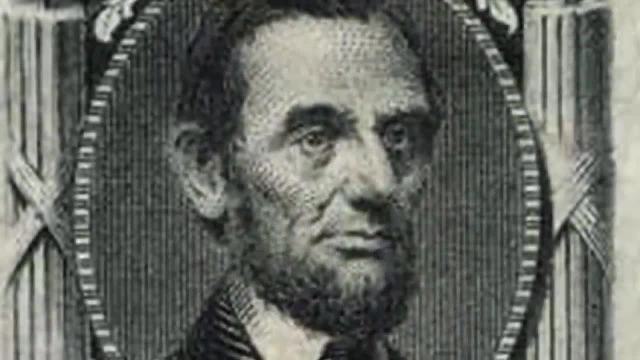 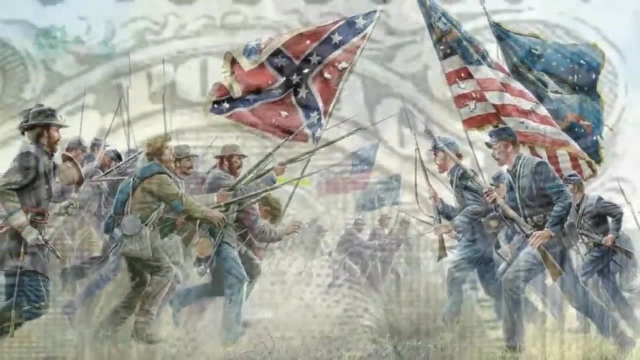 vertical ridges which were a standard feature. The face of the 16th president looking to the right on the horizon. Its rarity is due to the issue of the stamp during the Civil War period. at the top, the numbers representing the face value of the stamp- 15 cents- while at the bottom, the 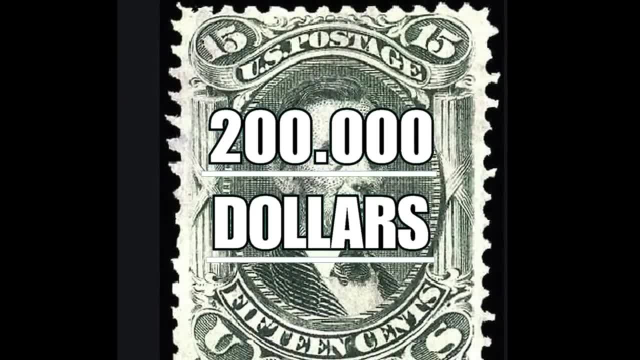 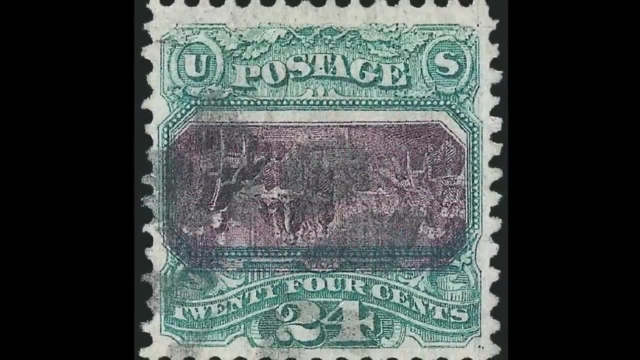 number written in letters. One of these can be worth around $200,000.. The 24-cent Declaration of Independence stamp has a unique rarity, namely the stamp is reversed Above the word postage. in the central part, the famous painting representing the Declaration of Independence. 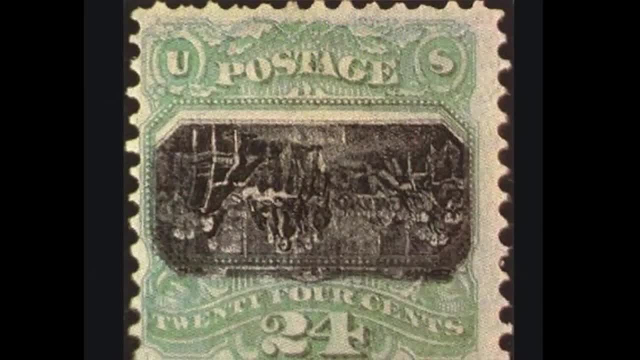 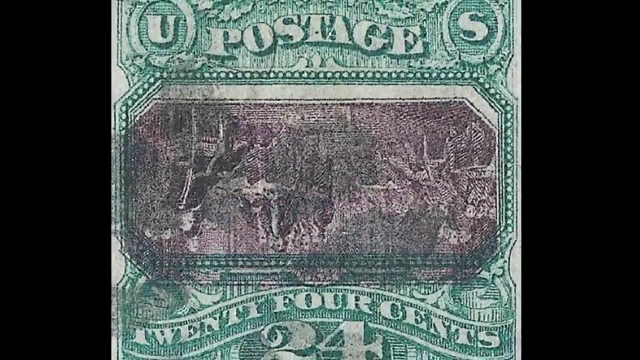 signed in 1776.. If you have an unused sample with an inverted center, it is estimated that you will have a stamp of the same value. The stamp is a unique rarity, namely the stamp is reversed. The stamp is a stamp worth $275,000 on hand. The Columbus Landing stamp, printed in 1869, represents 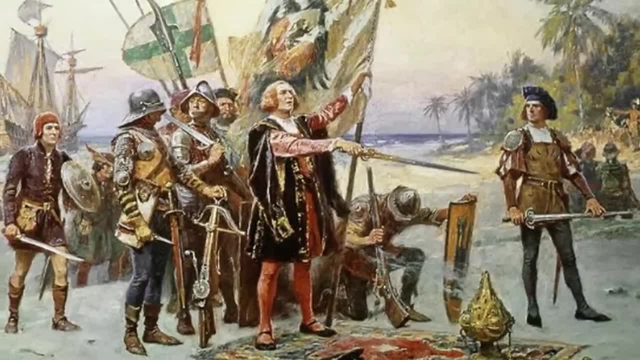 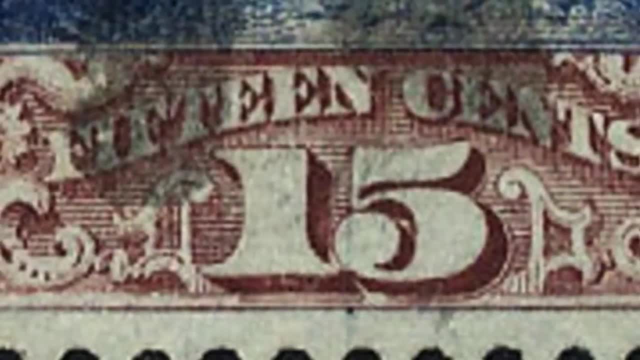 the discovery of the American continent by the European Christopher Columbus. Its rarity is the unusual double-printed vignette with normal and inverted printing applied Under the figure the writing 15 centesimi above the writing postage. An inverted sample of this stamp, when sold at: 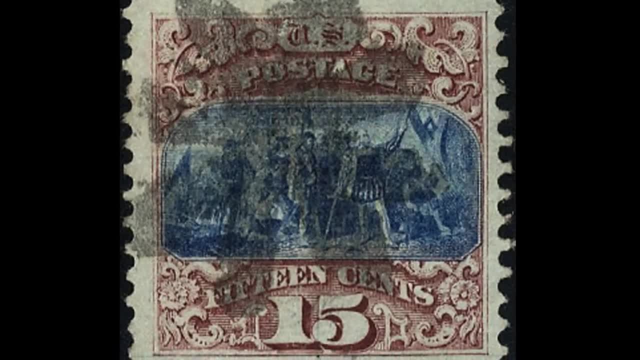 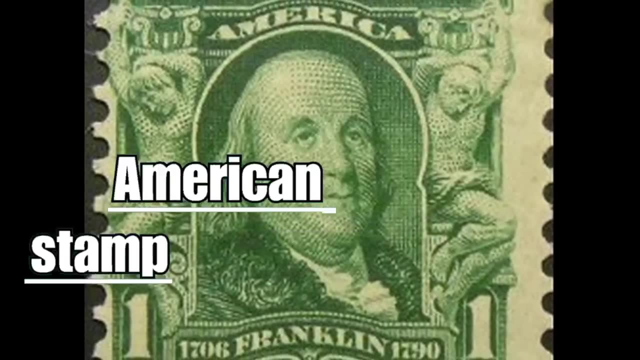 auction can be worth up to $280,000.. The 1C Benjamin Stamp is a stamp of the American continent and is considered to be the rarest and most expensive American stamp. Issued in 1867, it represents the 6th President of the United States of America, famous scientist in many.